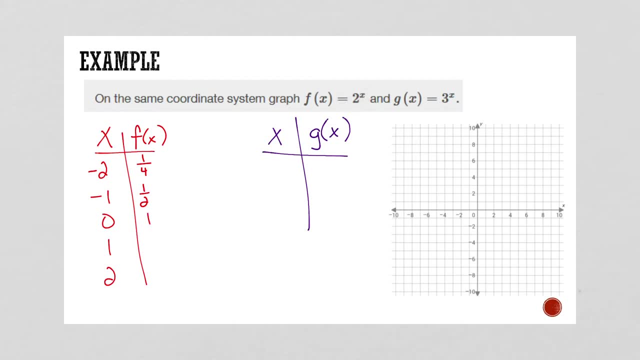 2 to the 0 power. remember: anything raised to the 0 power is 1.. Then if I put 1 up in the exponent, 2 to the first, power is just 2, and 2 up in the second, up in the power, then I've got 2 squared, which is 4.. 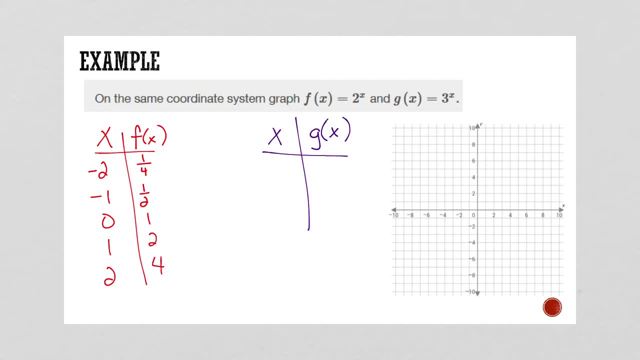 Okay, so let's graph these. So negative 2 and then 1 fourth is our y. So negative 2 and 1 fourth are our y. So negative 2 and 1 fourth are our y. So negative 2 and 1 fourth are our y. 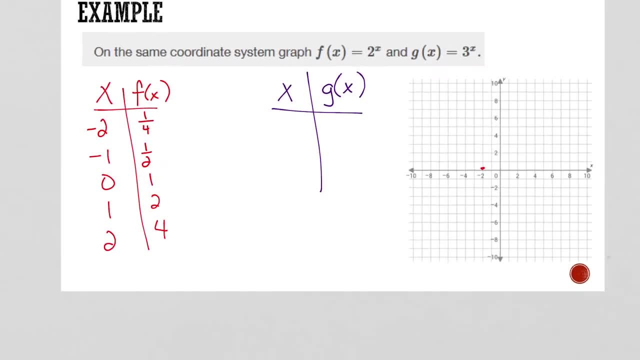 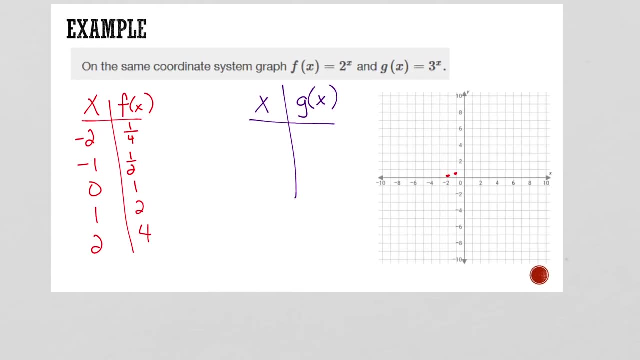 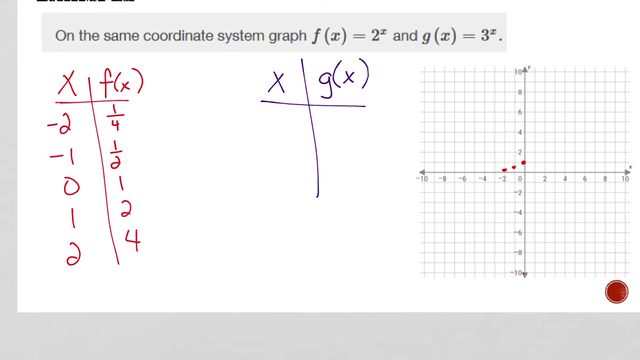 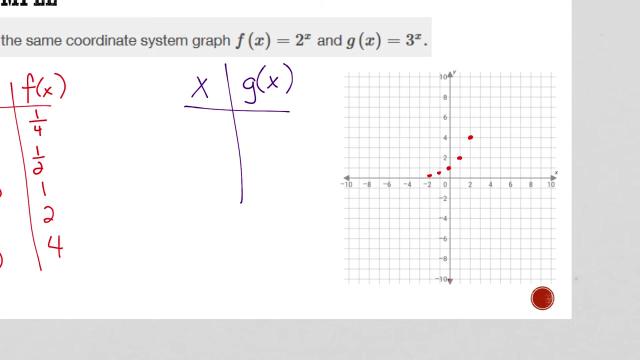 That's approximately right there. Then I've got negative 1 and 1 half, which is about there. Then I've got 0 and 1, which is right there- Make this graph just a little bit bigger- And then we have 1 and 2, and then 2 and 4.. So our graph actually looks like this: 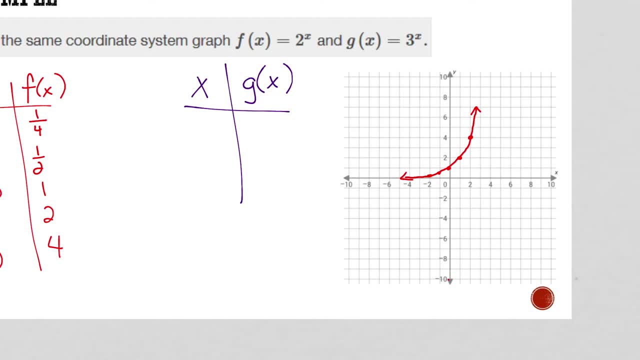 That's usually what an exponential graph looks like. It's curved and it'll take a very sharp turn upwards. If it's a negative number, it goes like this: Okay. but if it's a positive number- this number, I mean the base- then it goes like this: But we're not going to worry. 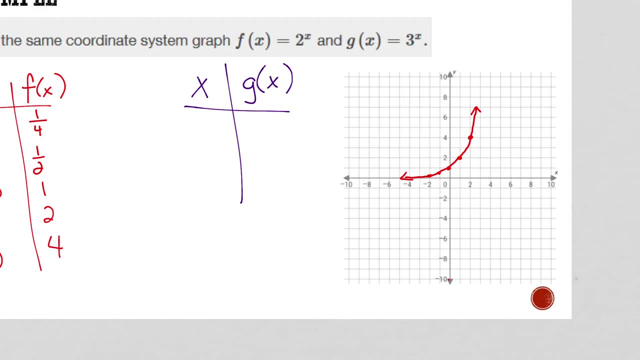 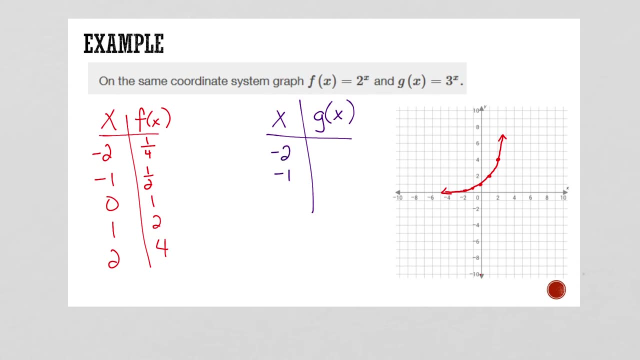 about that right now. Okay. so let's start with the same numbers for x here. So we're going to start with the same numbers for x here, Okay. so if I put negative 2 in the exponent, that's the same thing as 1 over 3 squared, which is 1 over 9.. If I put negative 1 up in the 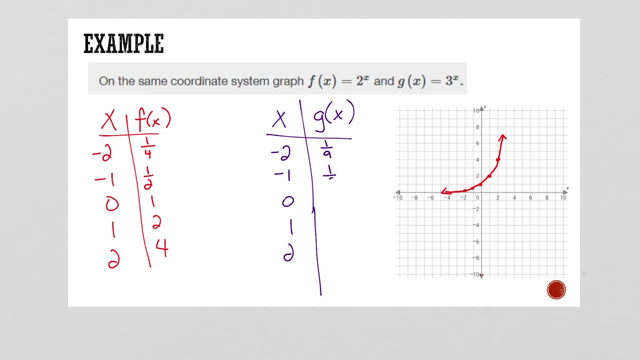 exponent, I end up with 1 over 3.. If I put 0 up in the exponent, I end up with 1.. If I put 1 in the exponent, I end up with 3.. And if I put 2 up in the exponent, I end up. 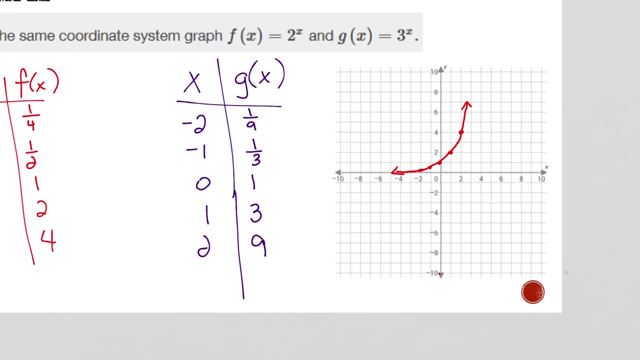 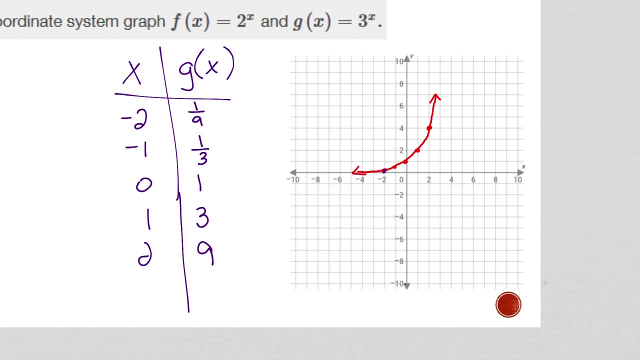 exponent, I end up with nine. All right, let's graph this now in purple Negative: two, one-ninth, So that's even closer to zero, but not exactly One-third would be about there, so it's slightly below this. They both go through this same point right here. One and three goes right here, and 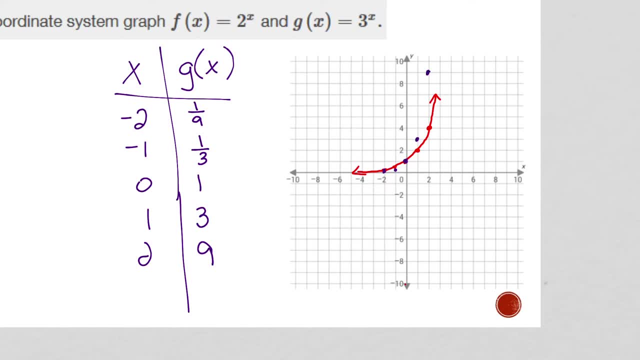 then two and nine is up here. Okay, so this one looks very similar, and notice that they both go through this point right here. That's what you're going to find is very similar on all of these, because anything raised to the zero power is one, so all of your exponential graphs will go through. 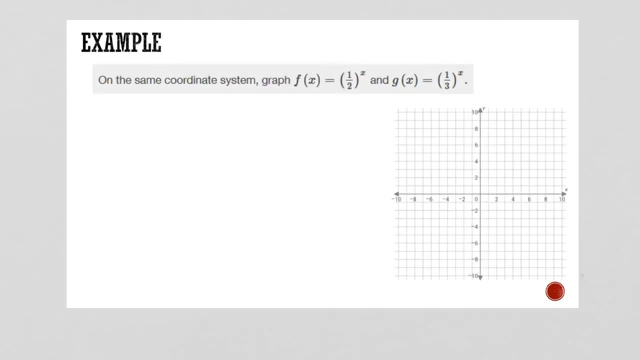 zero and one. All right, let's do the same thing with these problems now. Very similar to the last one, except now we've got fractions as our base. Ooh, let's see what happens with those. So we've got- oh, here I'm going to do- function notation. 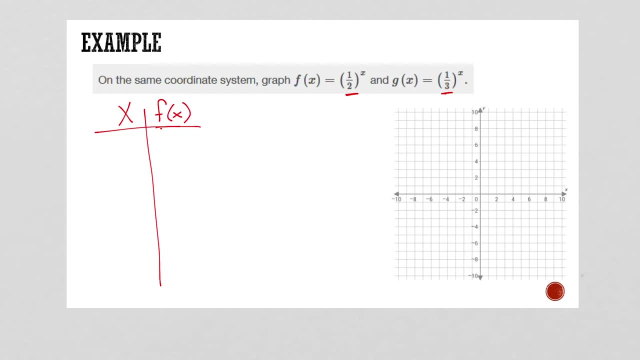 because that's what they're using. Okay, so we have. let's see here, Let's do the same ones again. Oh, there we go. Okay, so I've got one-half raised to the negative 2 power. That means I have, and I'm not going to do this for all the problems, but I do want to. 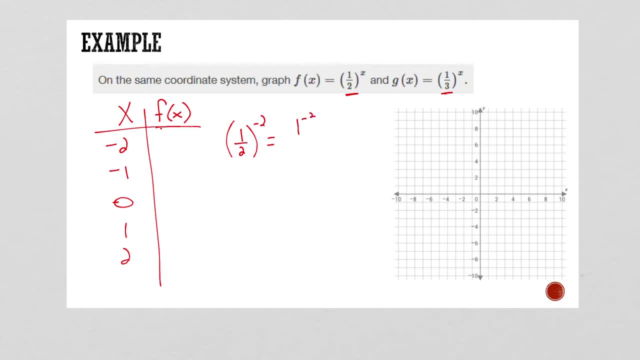 show you at least this first one. That means I have 1 to the negative 2 power and I've got 2 to the negative 2 power. Flip-flop their places because, remember, the negative exponent means they don't like where they're located. So this would be just 4, okay. And then, whenever I do, 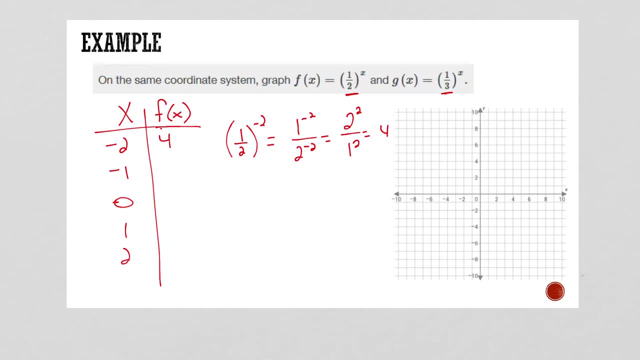 the same thing with negative 1, I'm not going to really go through that math, but you end up with 2.. Anything raised to the 0 power is 1. 1, 1 half raised to the first power is just 1 half. 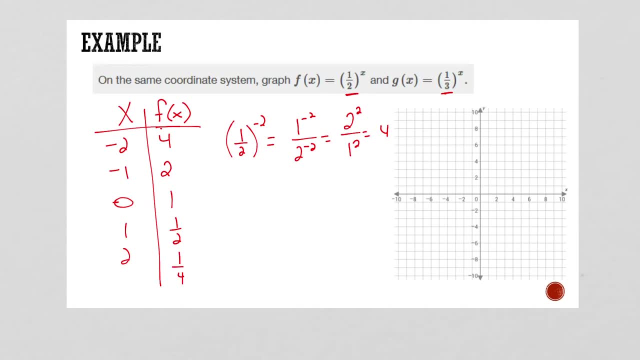 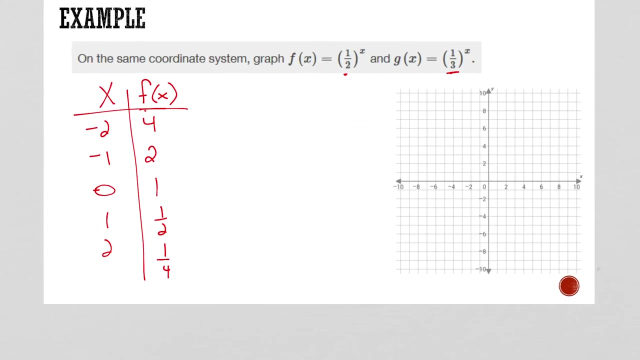 and then 1 half raised to the second power is 1. fourth: Okay, so I'm going to go ahead and erase this work right here, so if you don't have it written down, you should get it that way. Okay, now let's graph this: Negative: 2, 4.. 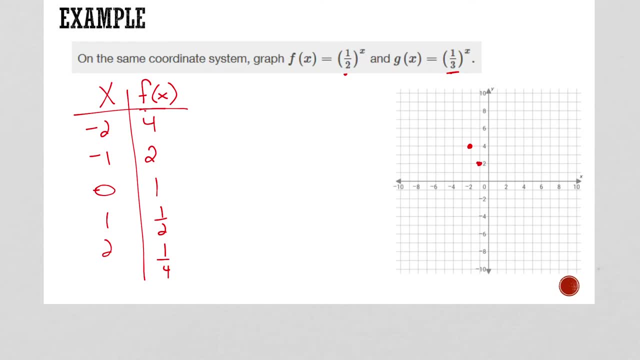 Negative: 1, 2.. Ooh, look at that. Look what's happening on this one: 0, 1.. Notice it still goes through 0, 1.. 1 and 1 half is right there, and then 2 and 1 fourth is right here. Okay so, 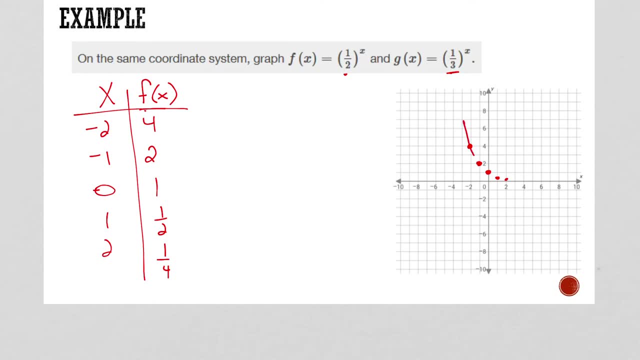 notice that whenever our base is a fraction, it goes in the other direction. I think I misspoke earlier. I said that a negative number would make that happen, and that's wrong. When your base is a fraction or a number between 0 and 1, then that will give you that. 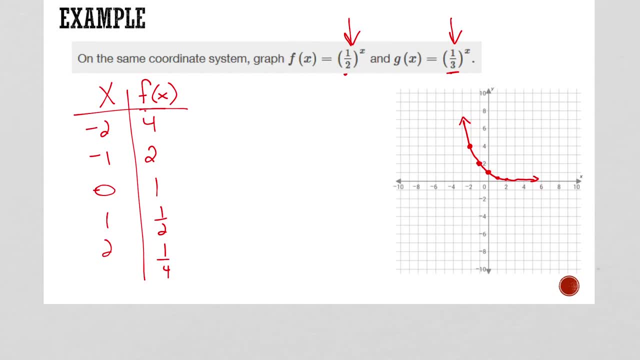 downward trend like that. All right, let's take a look at the g of x problem. All right, so let's use those same numbers. Okay, we know that this one's going to be 1, right, Okay, so whenever we have. 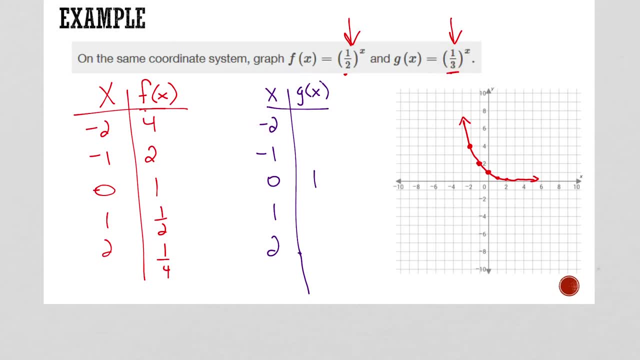 this raised to the negative 2 power. remember that makes everything swap, so we end up with 9.. And then to the negative 1 power: we end up with 3.. To the first power, we end up with 1. third, 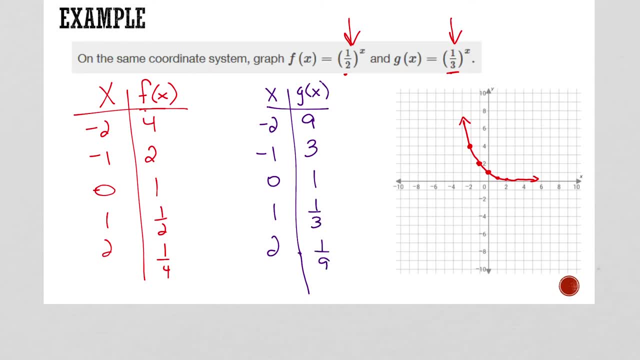 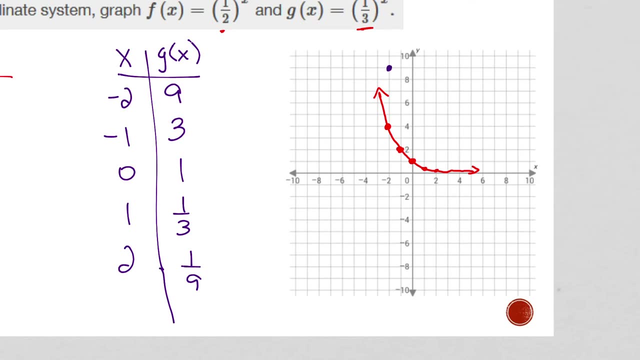 And to the second power, we end up with 1 ninth. All right, let's graph that. Negative 2, 9 is right there. Negative 1, 3 is right here. 0, 1 still goes through that spot. 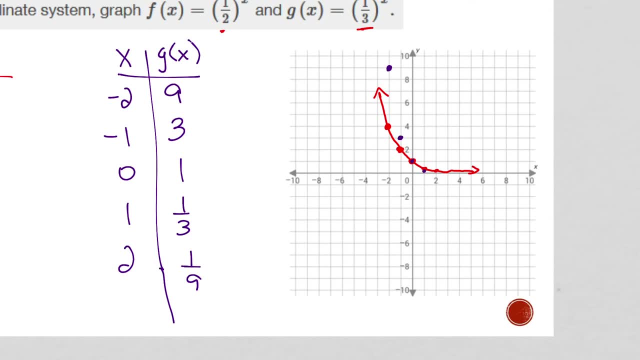 1 and 1 third down here, And then 1 and 1 ninth is way close to 0,, but not quite 0.. By the way, this will never, ever cross this x-axis. You can keep putting in numbers all day. 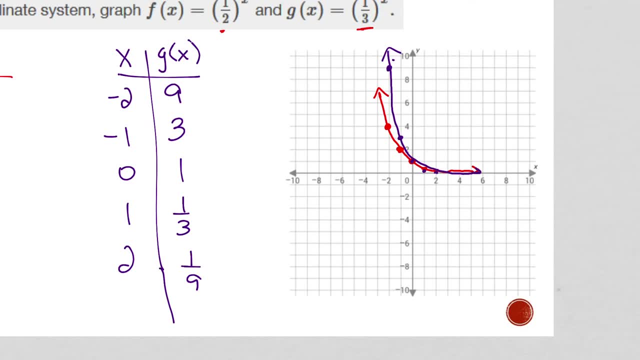 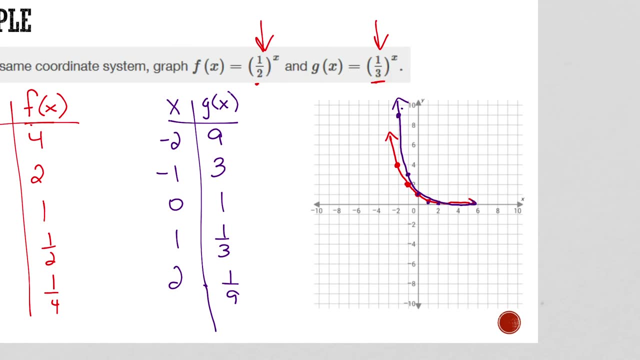 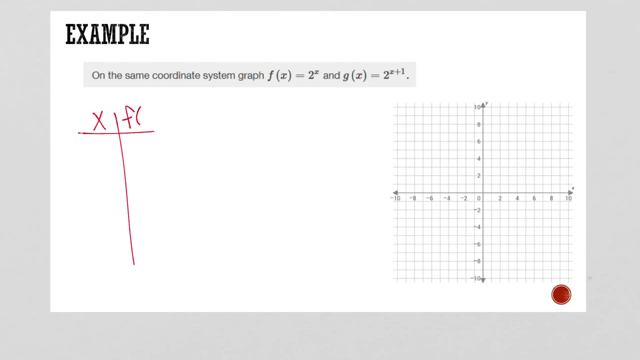 long and you will get super-duper close to 0, but you will never, ever cross that x-axis in an exponential function. Okay, let's do another, the one, Alright, so let's do. let's see here x and then f of x. Let's do the same numbers. 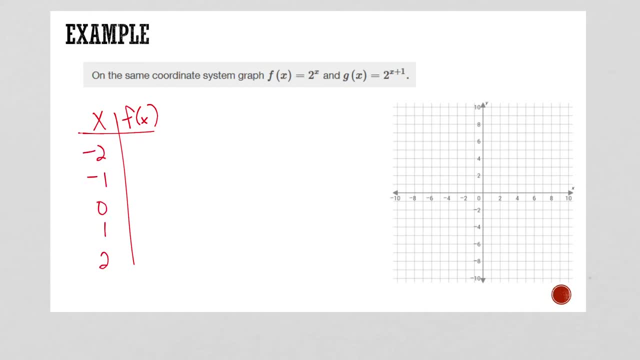 that we've been using. Okay. so whenever I put in negative 2, oops, hold on negative 2 right here. 2 to the negative: 2 is 1 fourth. 2 to the negative: 1 is 1 half. We did this. 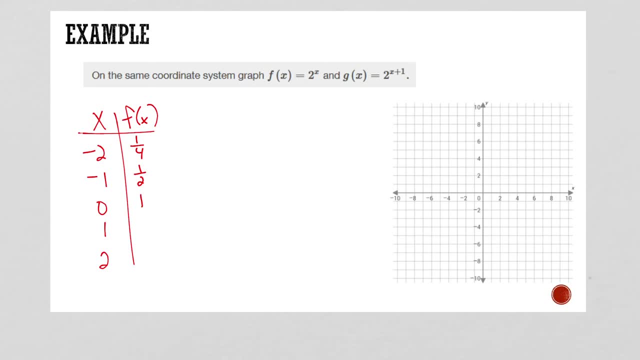 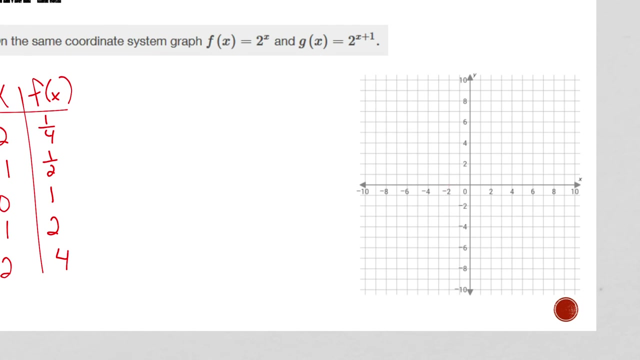 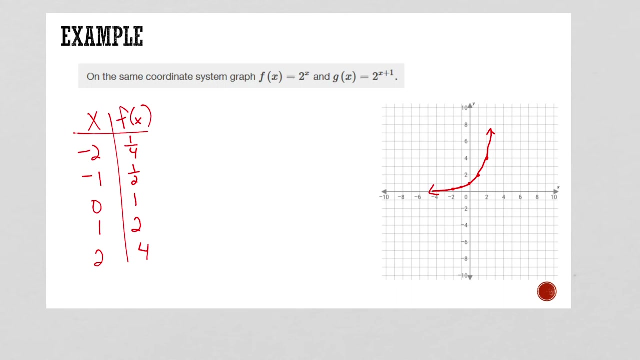 one earlier. so I'm just rewriting what we have. Alright, now let's see what the difference is between this and whenever we add 1 in that exponent. So let me go ahead and graph that real quick. Alright, now let's do x and then g of x. Alright, do the same numbers here, Alright. 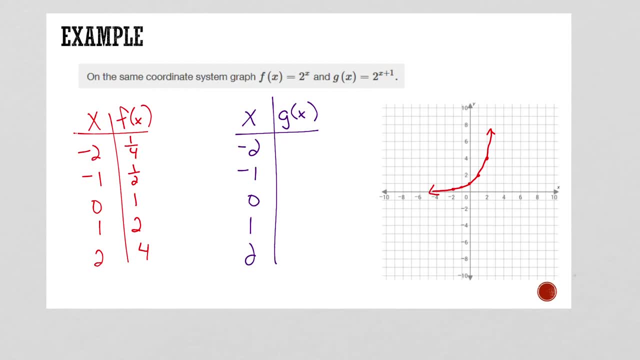 so now we've got- let's see here I'll do the math up here- 2 to the negative, 2 plus 1, which is 2 to the negative 1 power, which is 1 over 2.. Okay, 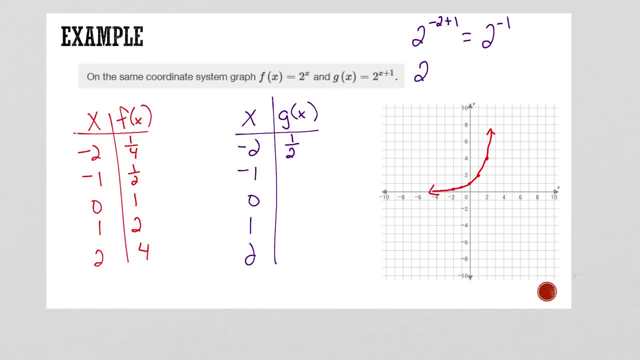 so now let's do the same thing up here: 2 to the negative, 1 plus 1, which is really 2 to the 0,, which is 1.. Now, 2 to the 0 power plus 1 is really 2 to the first power. 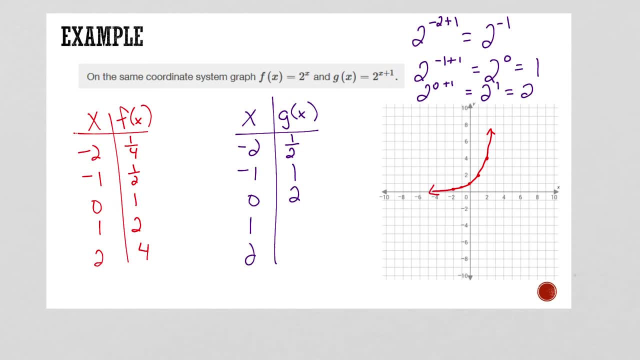 which is 2.. Now if we substitute in 1, right there, 1 plus 1 is 2,, 2 to the second power is 4.. And then if we do 2 to the 2 plus 1, so that's 2 to the third power, which is 8.. 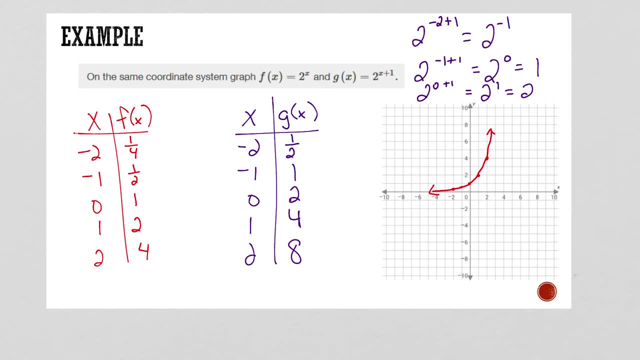 Alright, so negative: 2, 1 half. Okay, So slightly above. I love that one. Negative: 1, 1.. Ooh, look what that did. Now it won't go through 0, 1,, will it? 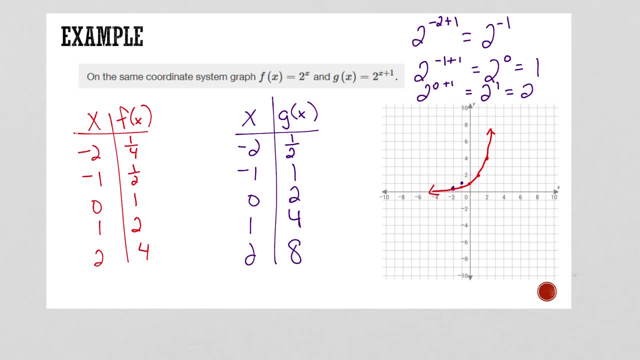 We had scooted it to the left right. Okay, 0, 2,. so now it goes through: 0, 2.. And then 1, 4. And 2, 8.. Alright, so look, here's what we've discovered. Whenever you're adding or subtracting up here, 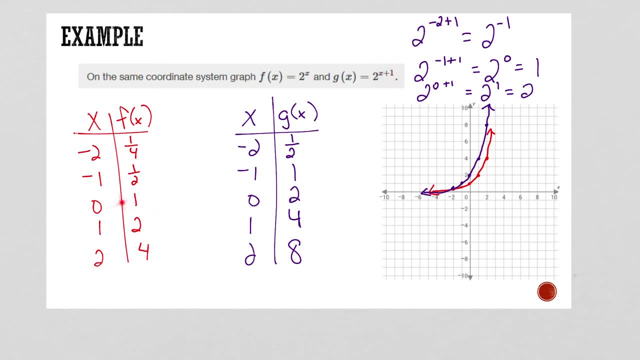 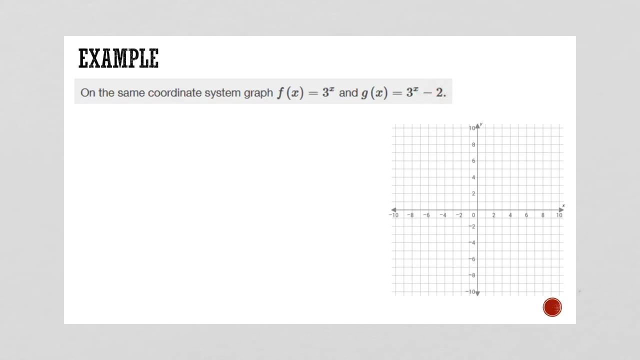 in the exponent, then you don't go through 0, 1 anymore, do you? So that's only if you have just plain old x up there do you go through the 0, 1.. Okay, so what happens whenever we don't have the minus or a plus in the exponent? It's: 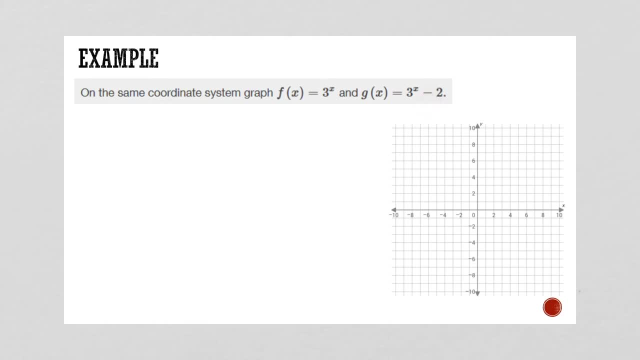 now down here. Hmm, let's see what happens. Alright, so let's do the first one. So whenever I put in negative 2 right here, 3 to the negative 2, power is 1, 9th, 3 to the. 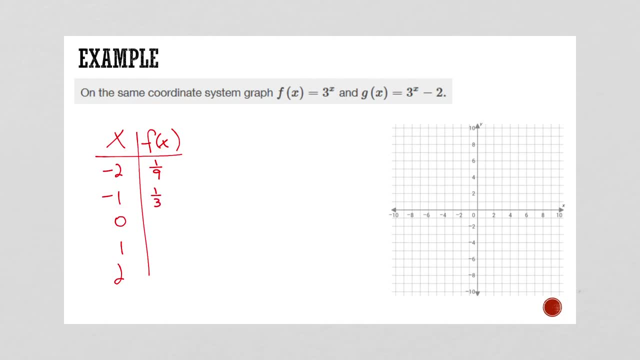 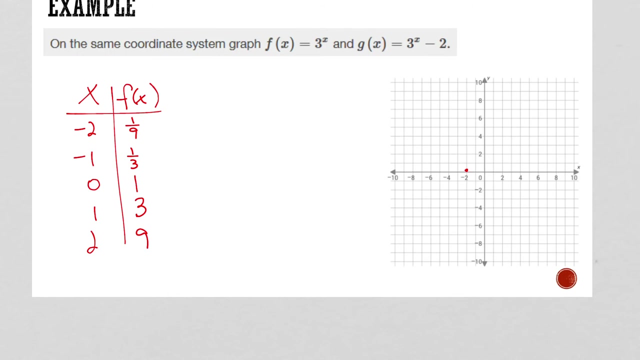 negative: 1 power is 1. 3rd, 3 to the 0 power is 1,. 3 to the first power is 3, 3 squared is 9.. Alright, let's graph that. I don't know exactly where 1- 9th is, but I do know that it's really really close to. 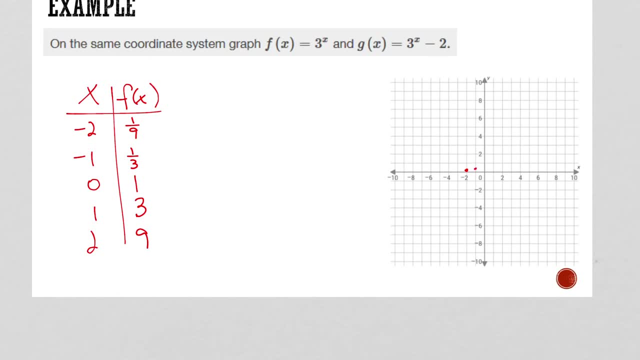 0.. Negative: 1, 1. 3rd, slightly above that: 0, 1 is right there. 1, 3 right there. 2, 9 is up here. By the way, Whenever you do your homework online, you only need two points to graph. okay. 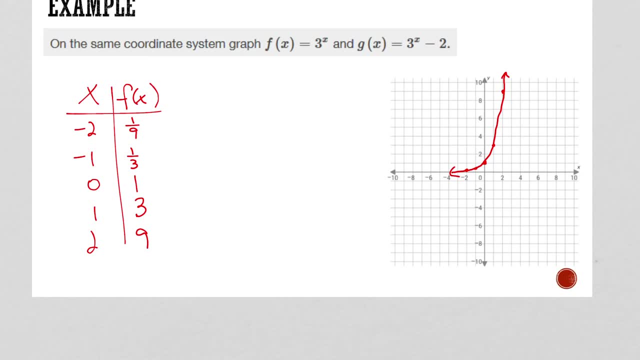 If you try to put any more than two points on your graph, it will mark it wrong. So make sure that you use any two of your points, Like I usually would use these two. right here I would use those two points and then I would spot check with those other three. 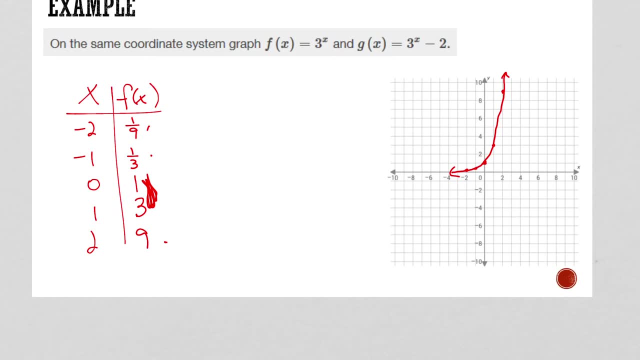 Alright, let's do the g of x now. Okay, Okay, Okay, Okay, Alright. so let's do the same numbers. So if I have 3 to the negative 2 power minus 2, okay, So 3 to the negative 2 power is 1, 9th minus 2, which would be 1, 9th minus 18 over 9, because 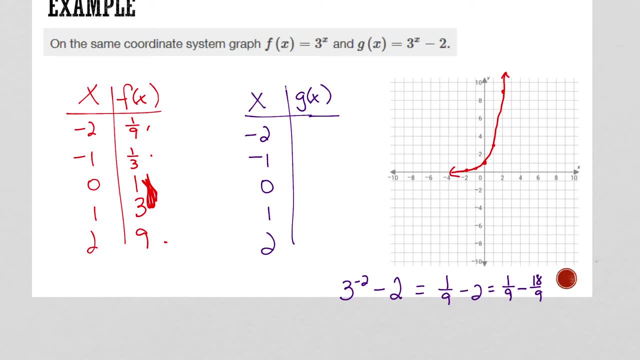 that's my common denominator. So I get negative 17 9ths- which, by the way, negative 17 9ths would be about negative 1- and 8 9ths, which is basically negative 2.. Alright, let's do the same thing for negative 1.. 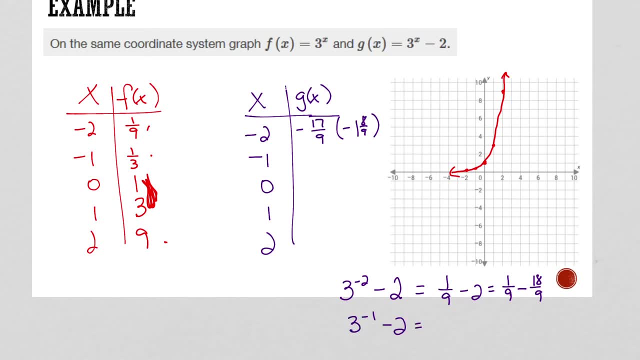 So I've got 3 to the negative 1 power minus 2, so that would be 1 3rd minus 2, which is 1 3rd minus 6 over 9.. Okay, So I've got 6 over 3, negative 5 over 3.. 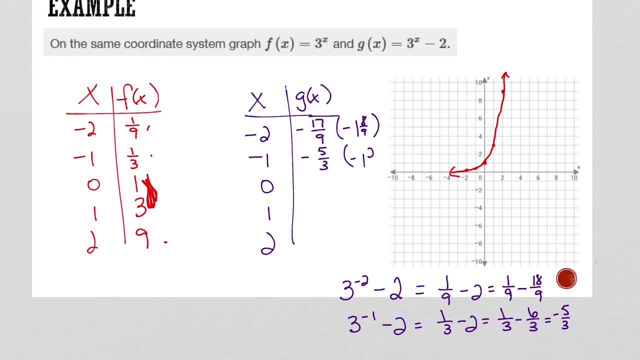 Negative 5 3rds, which is the same thing as negative 1 and 2 3rds. Alright, so if I raise that to the 0 power, so I've got 3 to the 0 power minus 2, which. 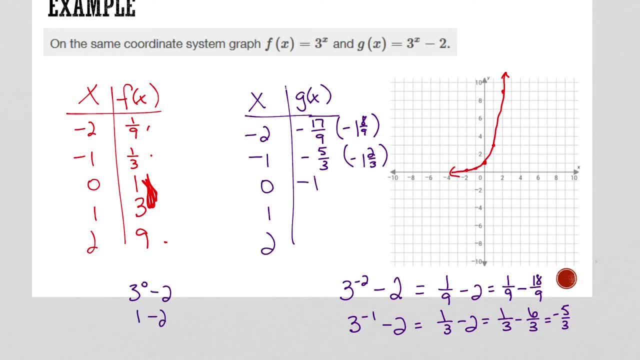 is 1 minus 2, which is negative 1.. And then I've got 3 to the first power minus 2,, which is 3 minus 2, which is 1.. Okay, And then 3 squared minus 2,, which is 9 minus 2, which is 7.. 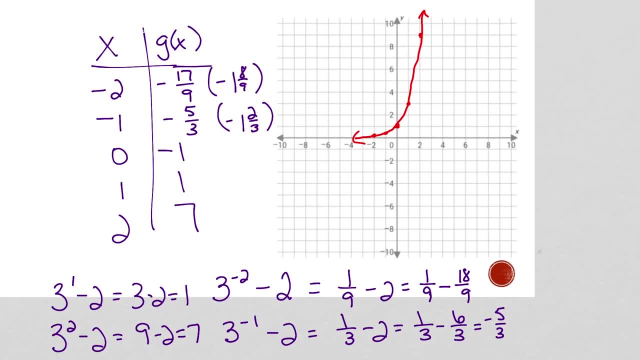 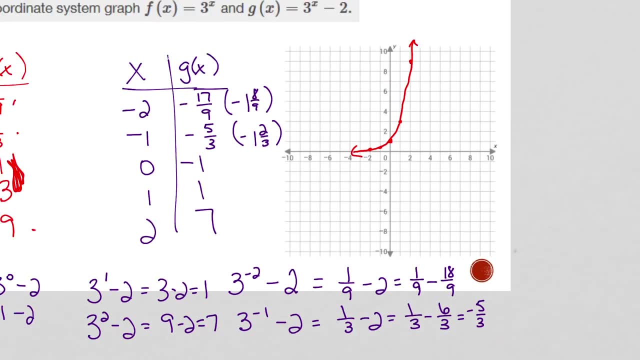 Alright, let's graph those. Okay, so we're going to graph this now. Okay, so negative 2 and negative 1 and 8 9ths. So negative 2 and negative 1 and 8 9ths. Oh, look at that. 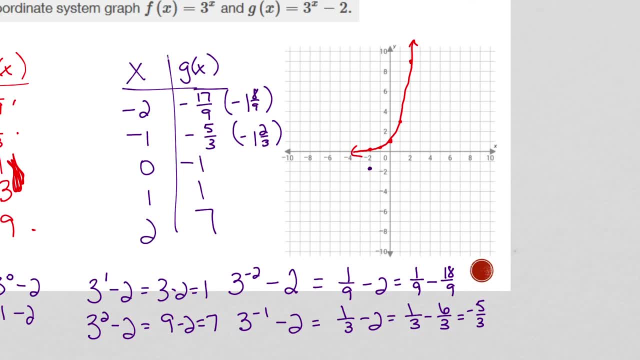 It took me a while. It took me a while. It took me a while. It took us below that x-axis. So what happens? What does this do right here? What does that minus 2 do? Moves things down, doesn't it? 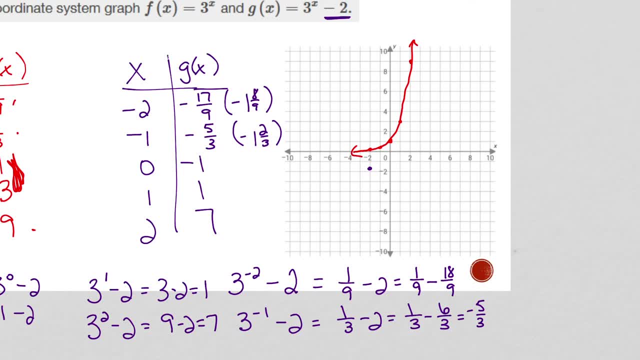 Okay. so now let's see here Negative 1 and negative 1 and 2 3rds- Okay, it's really going to be below negative 1 and 1 half, Okay. and then we've got 0 negative 1, which look at that. 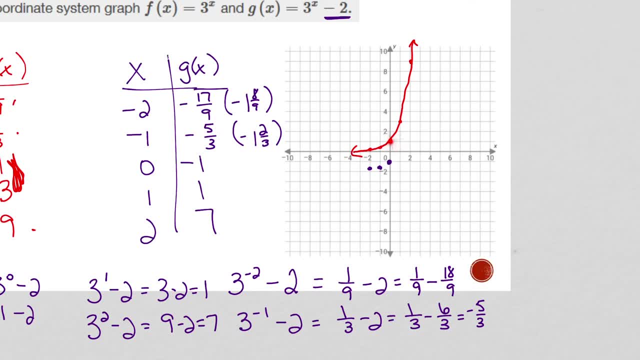 Negative 2, negative 1, negative 2, which are instead negative 1 and 2.. Yes, Negative 1 minus 2.. Next up is median Negative 2 plus 0.. Negative 1 minus 2 plus 0 is positive. 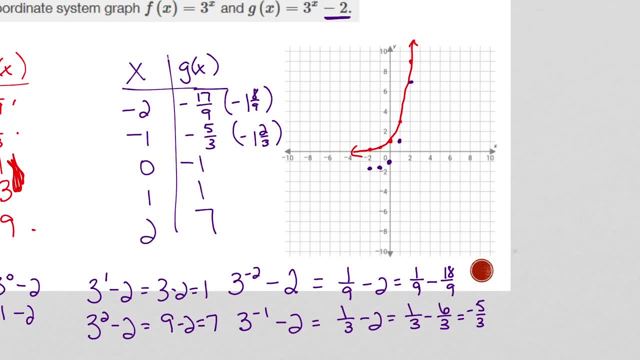 Negative 1 plus 2 is negative 1 plus 1.. all right, there we go. that's it again. when you're graphing, only use two points. i would probably use these two points, or these two, but only use two points, and then you spot check with the other. 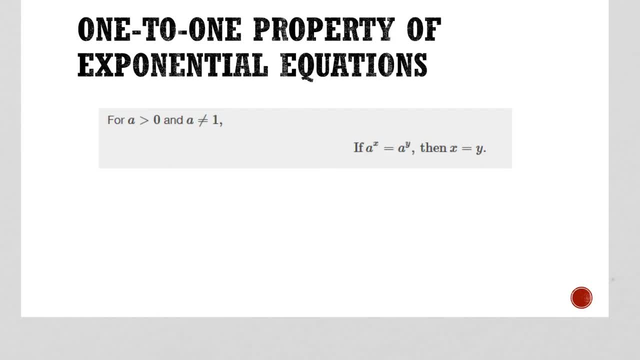 points. okay, so this page won't make a whole lot of sense to you until i show you some examples, probably all right. so it says your bases need to be greater than zero, so positive numbers, and it says that your bases cannot equal one. okay, so what it says is that if you have the same base, 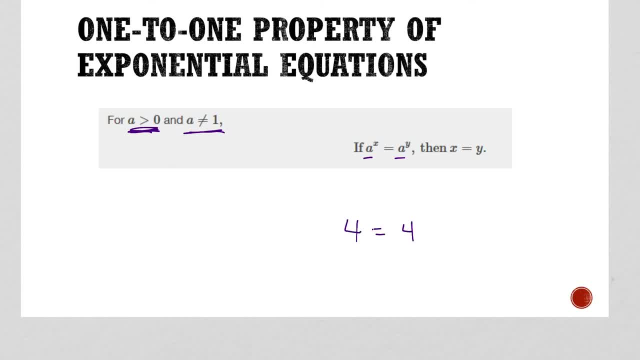 let's say we have four and we have four, and we have four to the x power is equal to four to the y power as long as your bases are the same. as long as your bases are greater than zero, but not one, then that means your exponents have to also be equal to each other. okay, and i'm going to show. 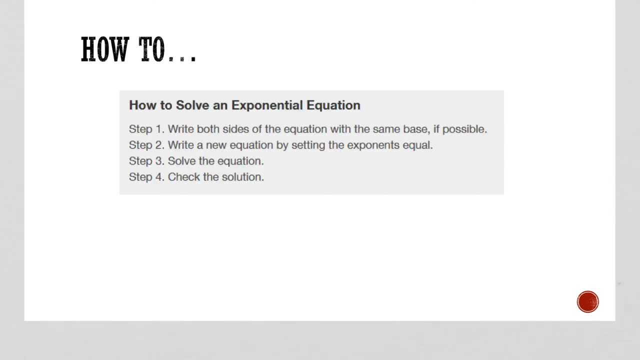 you what i mean here in just a second: how to solve an equation, an exponential equation. write both sides of the equation with the same base, if possible. okay, then write the new equation by setting the exponents equal to each other. solve the equation and then check your solution. 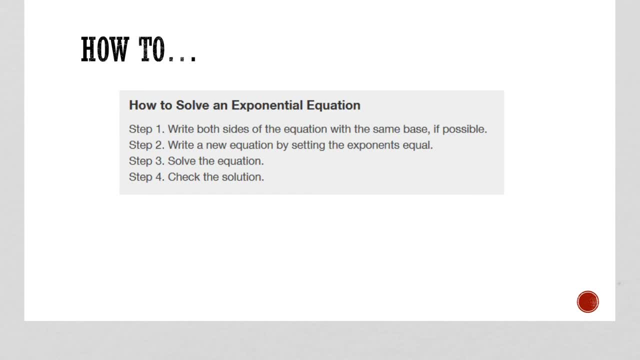 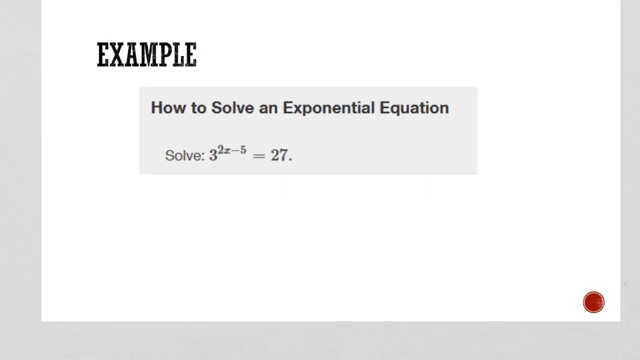 again. you don't have to memorize this, but you know just something you need to read through and see if you're following this. the steps again. this is significantly more difficult to um to solve for x because the x is in the exponent. okay, so here's what you want to do. you want to have the same base, so can we write this? 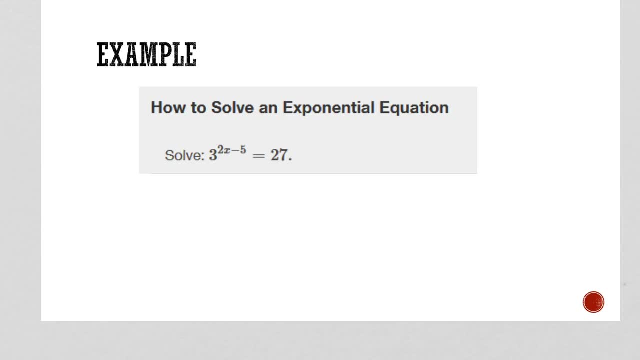 number as something with a base of three. yeah, we totally can. okay, so the left side, i'm just rewriting it. my right side, i'm going to write 27 as three to the third power. okay, as long as our bases are the same and the base is not a negative number or equal to zero, we're allowed to set the exponents. 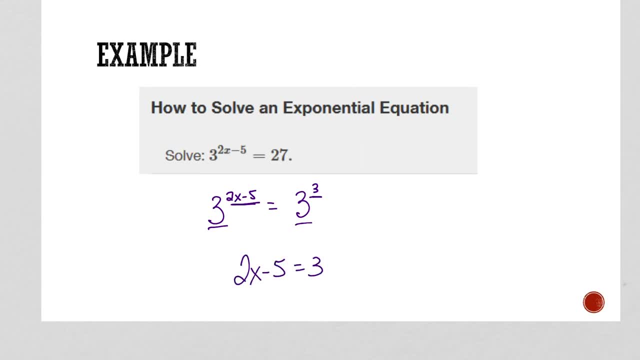 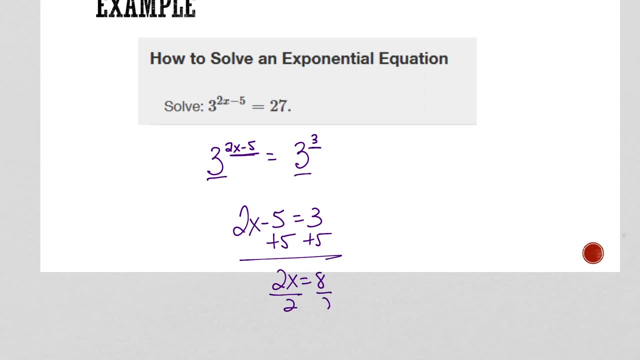 equal to each other, and now we just solve for x at this point. all right, so our x is four. can you check your work? totally, let's check it. so we've got three, and then we've got two times four minus five. does that equal 27? two times four is eight. 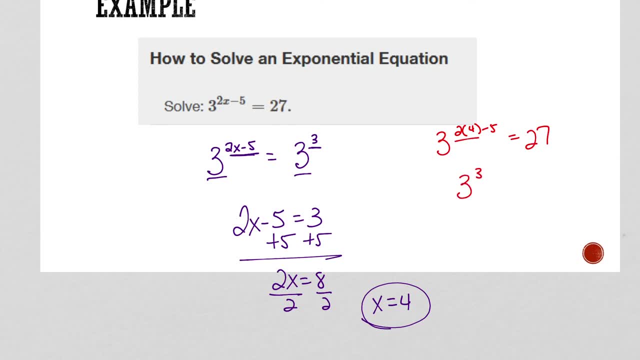 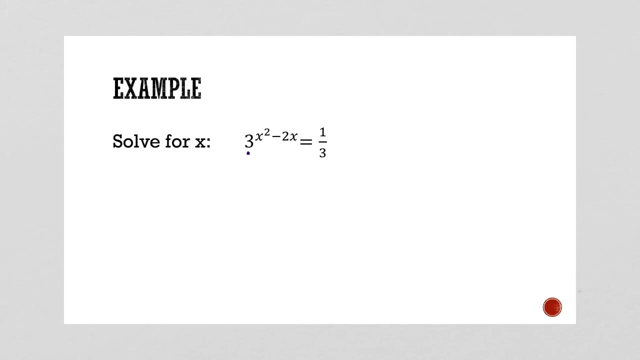 eight minus five is three is three to the third, power equal to 27. yep, 27 equals 27, so this is the correct answer. all right, let's look at this one. so we've got three to the x squared minus two. x equals one third. oh so can we write this as something? 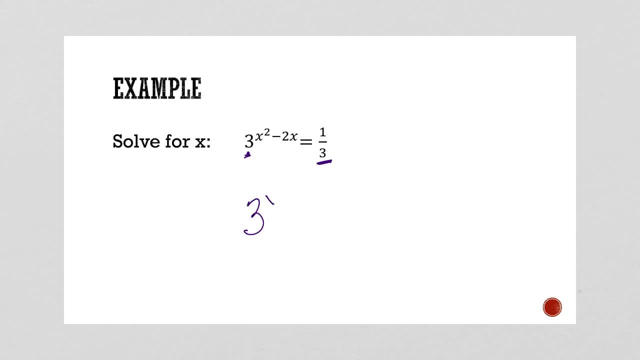 with a base of three. yes, we can. it would be three to the negative one power. okay, so now i've got this and this are equal to each other, and in order to solve for an x squared, remember, we're either gonna have to use the quadratic formula, completing the square, or we're going to need to factor. so i would pull everything. 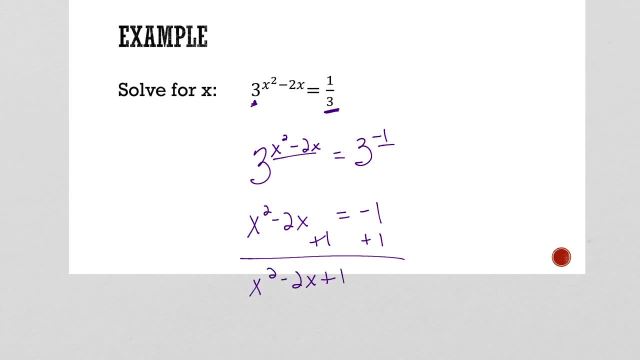 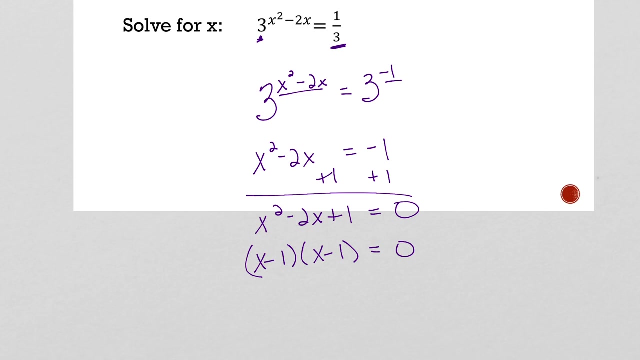 over to one side, and so this factors to be right, because it multiplies to be positive one, but it adds up to be negative two, and And I take that and set it equal to zero, So X is equal to one. All right, So now can we check our work. 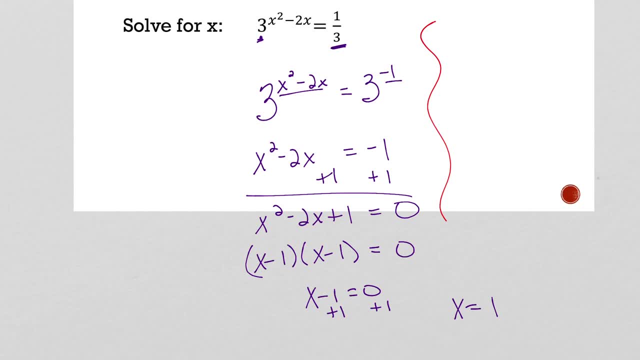 Yeah, we probably should too. All right, So we've got three to the one, squared minus two times one. Does that equal one third? I don't know. Let's see here: One squared minus two is So one squared is one.